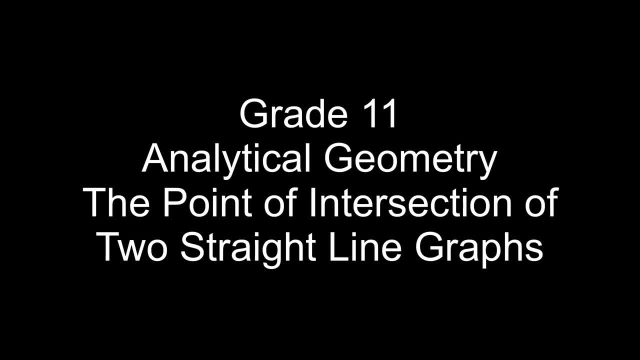 Hello grade 11s. Today we're going to look at the point of intersection of two straight line graphs. So if we think about it point of intersection between two straight lines, we've got a few options. The first option is if we look at these two little graphs at the bottom here. 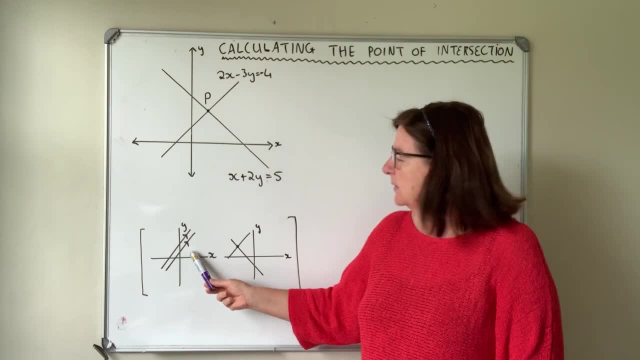 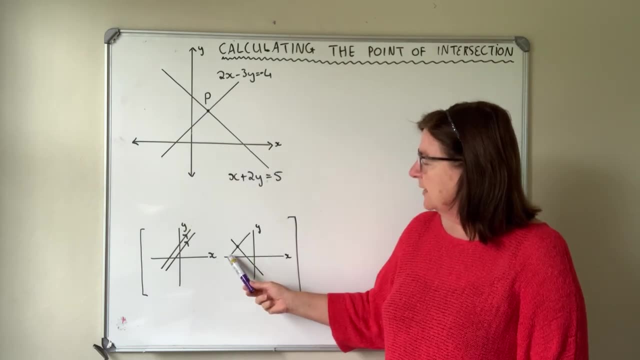 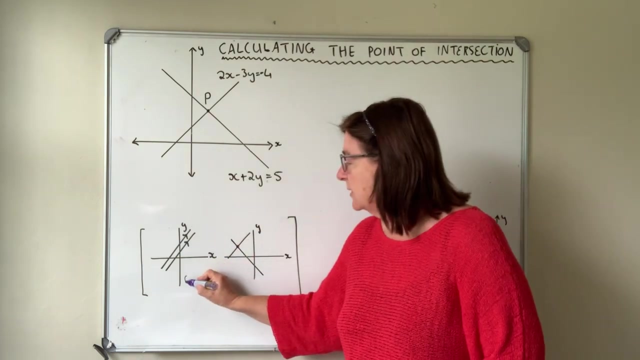 in that case, there, there's going to be no point of intersection because the two straight lines are parallel. And in this scenario, here there's one, two straight lines and they are only going to ever cut each other once. So they always, with straight lines, will either be zero points. 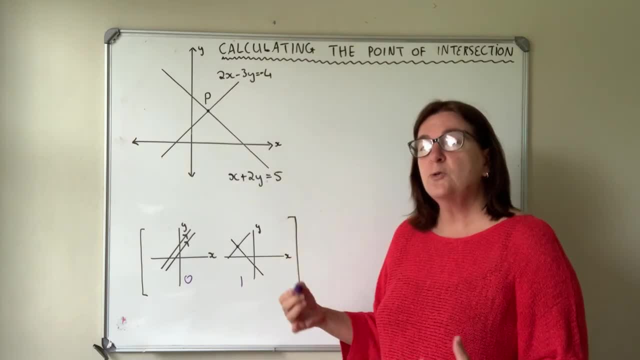 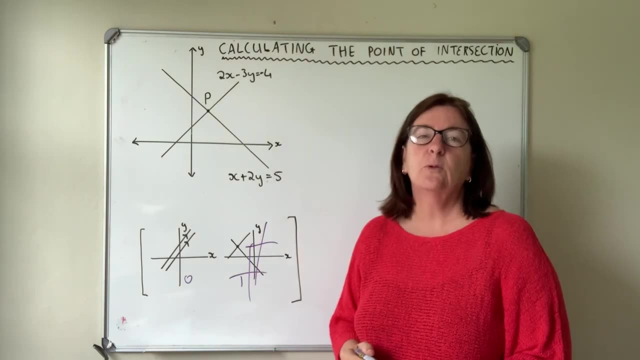 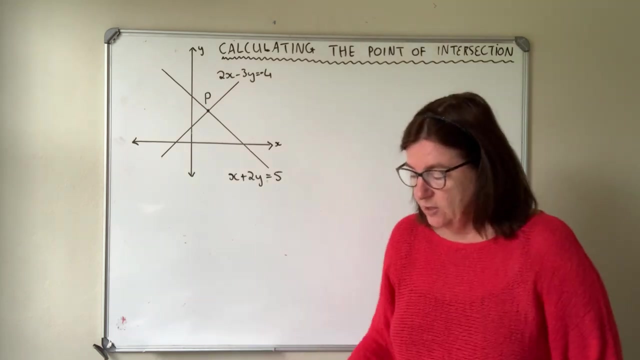 of intersection or one, Because irrespective of where we draw the two straight lines, because they continue in a straight line- there will always be only one point of intersection. Okay, let's quickly get rid of this. So now, the example that we're going to look at is this example: here We've got two straight lines with 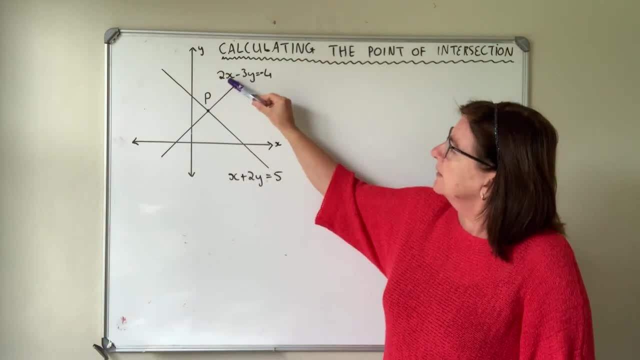 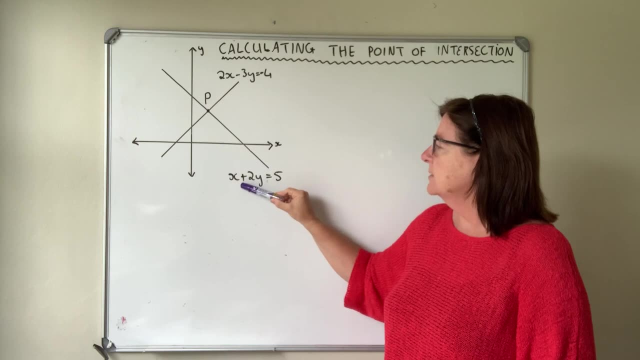 the given equation. So this straight line, 2x minus 3y equals minus 4, and this straight line is defined by this equation: x plus 2y equals 5.. Now the question is: we need to find that point. 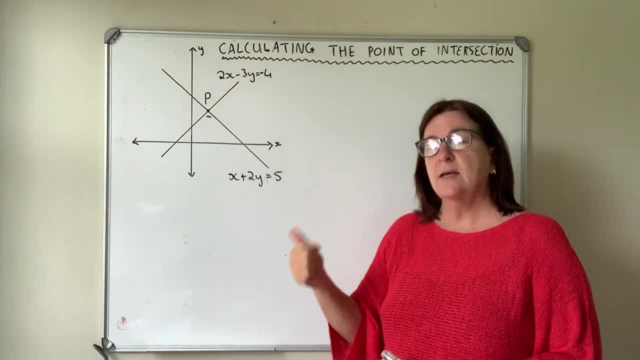 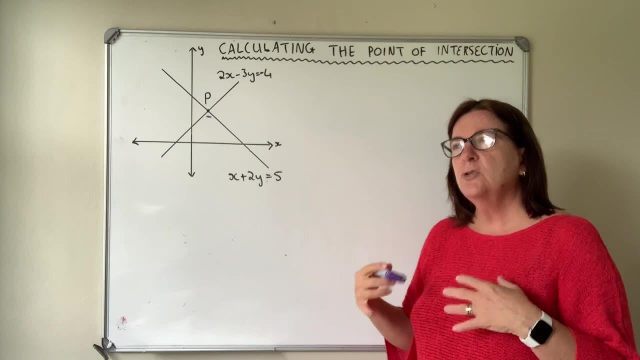 of intersection, which is p, It's going to have one x and one y because there's one point of intersection. Now, if we think back, how to solve this, when we've got two equations, two unknowns, we need to use simultaneous equations. This is 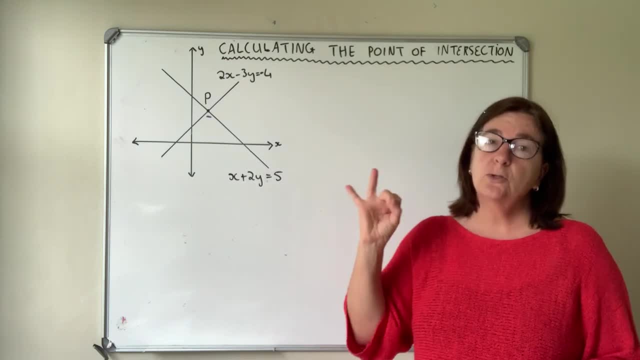 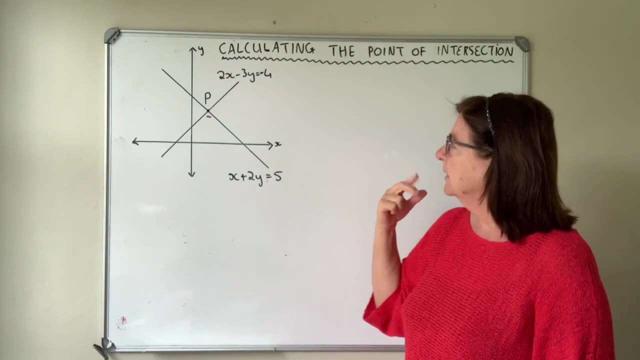 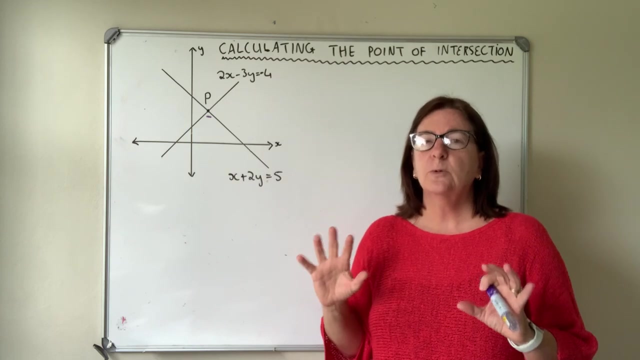 solving simultaneously. And remember there's always two potential methods. We have the substitution method and the elimination method, So we can always use one or the other, and it's completely up to you. You will always get the same answer, But I'm going to choose the elimination. 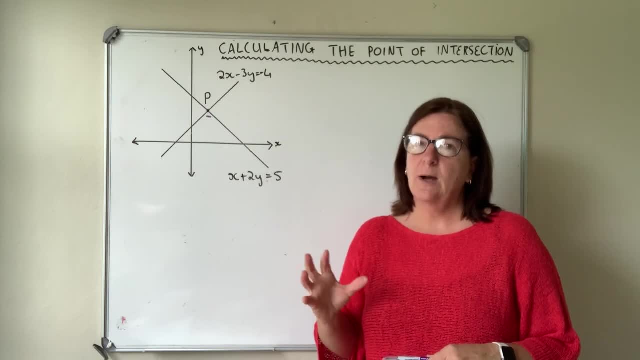 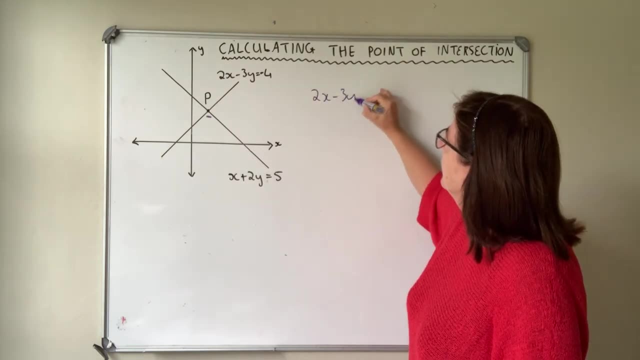 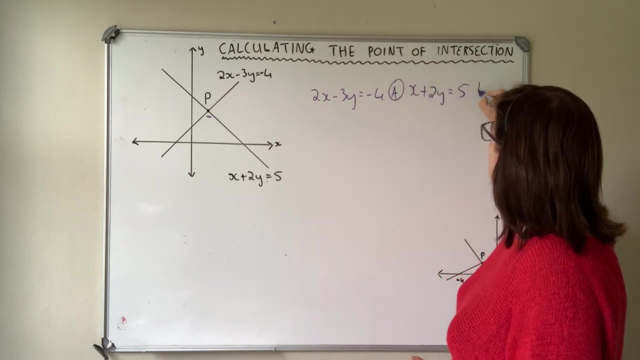 method here, because I've got straight lines x and y. I don't have an x and y, So I'm going to use the elimination method. So we've got our first equation And we've got our second equation. I'm going to call this equation A and I'm going to call this equation B. 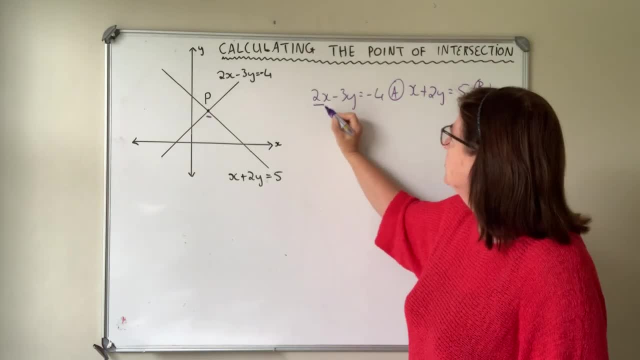 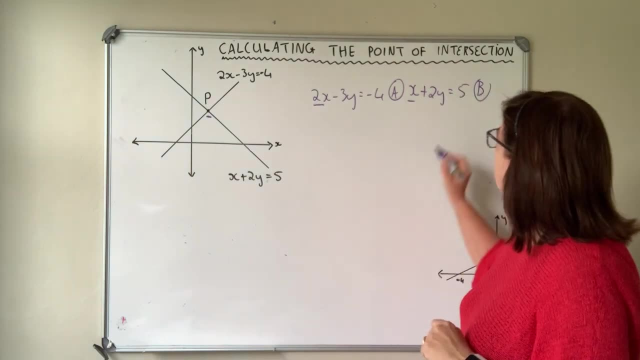 So now, if we look and we use the elimination, that coefficient is 2 and that is 1.. So they're different, So I can't eliminate. Remember they have to be the same. So I'm going to multiply equation B by 2.. So if I multiply I'm going to get the same answer. 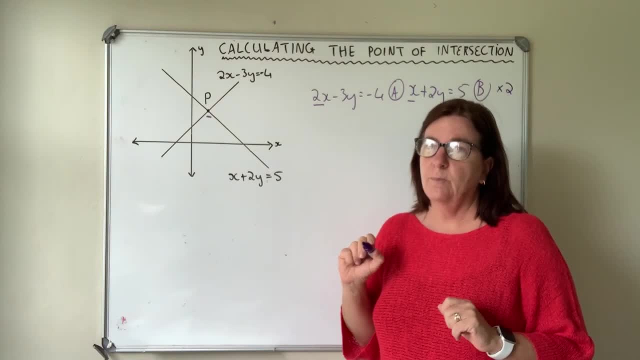 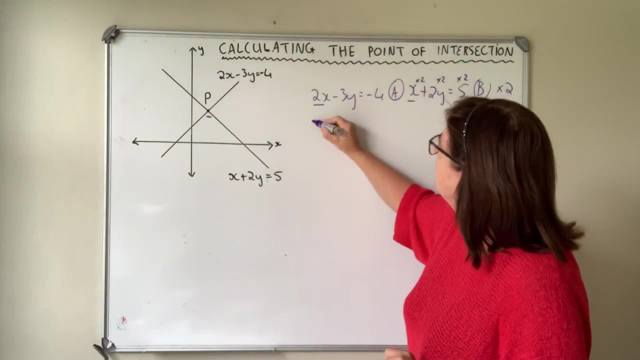 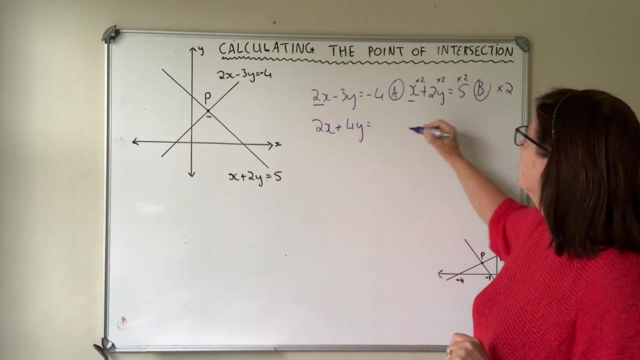 So if I multiply equation B by 2, I have to multiply every term by 2.. So that must be times 2, times 2, times 2.. So if I do that, I'm going to get 2x plus 4y equals 10.. And that's my equation. 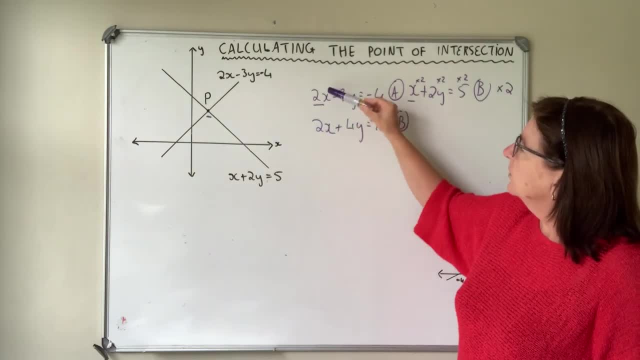 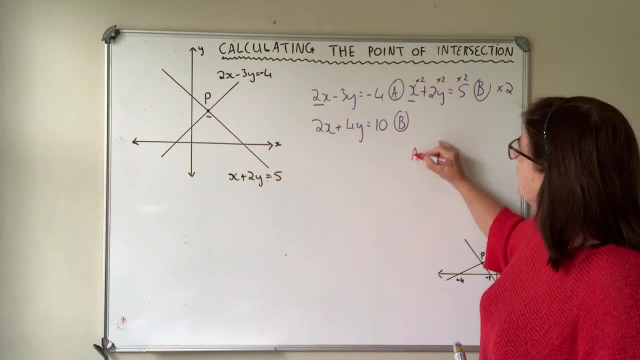 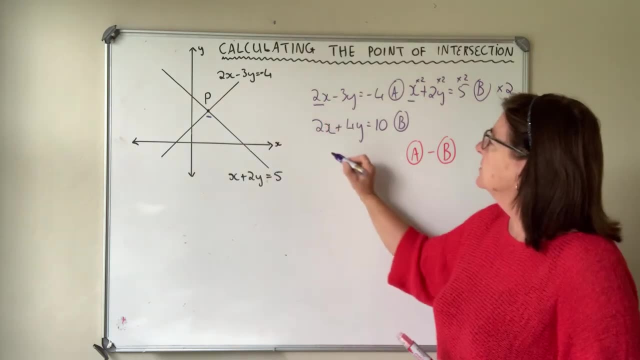 to do this. Do I add or do I subtract? So in this case, here we're going to have to do subtract 2x minus 2x. It's gone. The x's have been eliminated. Minus 3y, minus 4y is going to be. 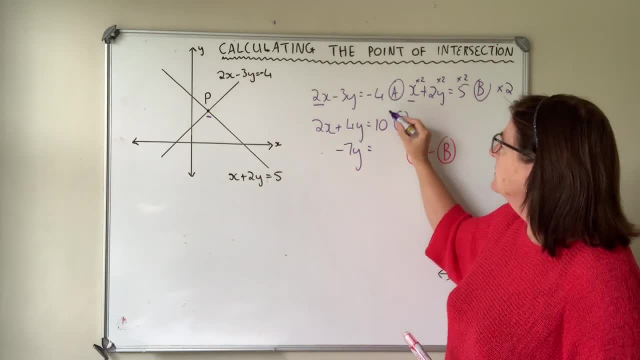 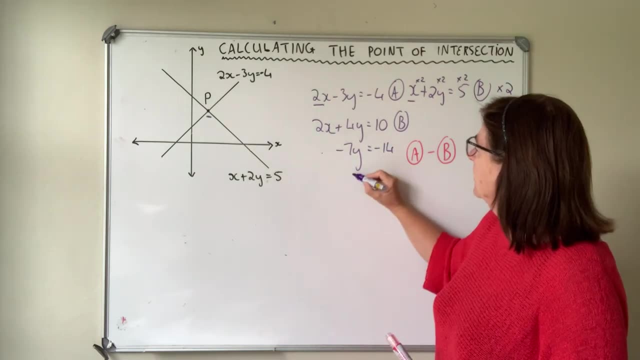 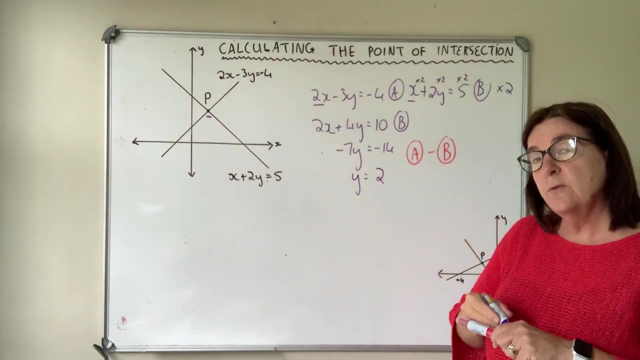 minus 7y Minus 4 minus 10 will be minus 14.. And now we've eliminated x, So we can solve for y. So y is going to be minus 14 divided Minus 7, which is going to be 2.. But we're not finished yet, because we've got y, Now we need to. 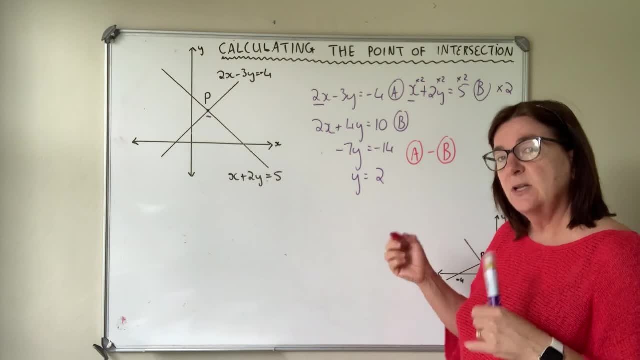 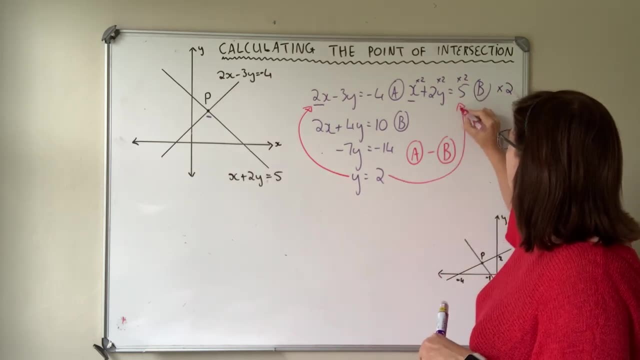 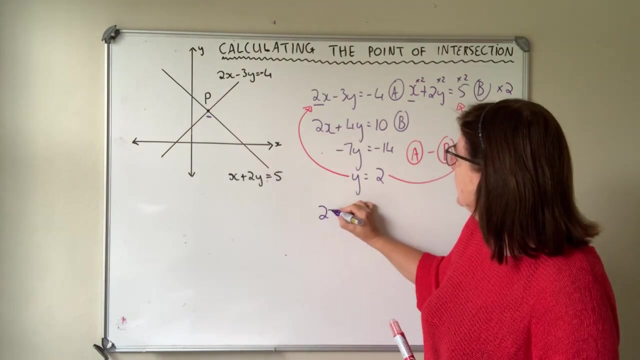 solve for x. So remembering, reminding ourselves back to elimination method, that y I can then substitute into either equation A or equation B- It doesn't matter which one, You will get the same answer. So I'm going to just sub it in here. So I'm going to get 2x minus 3y, But y is 2.. 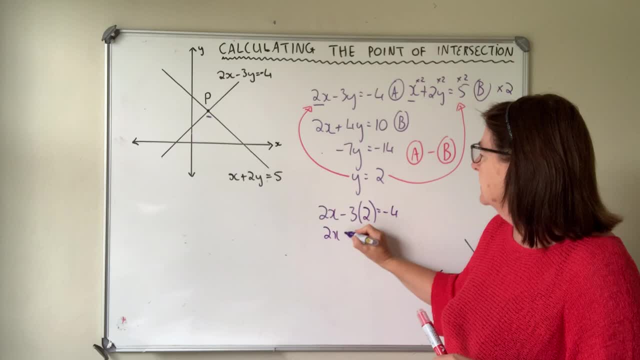 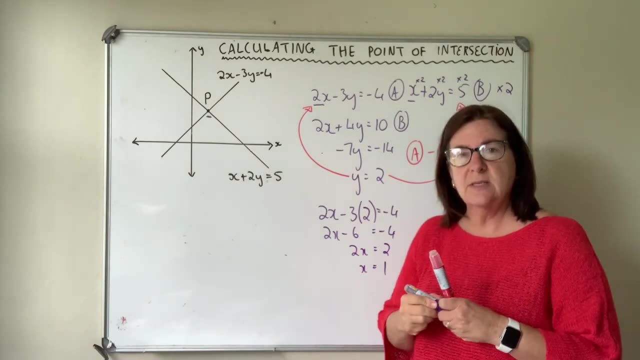 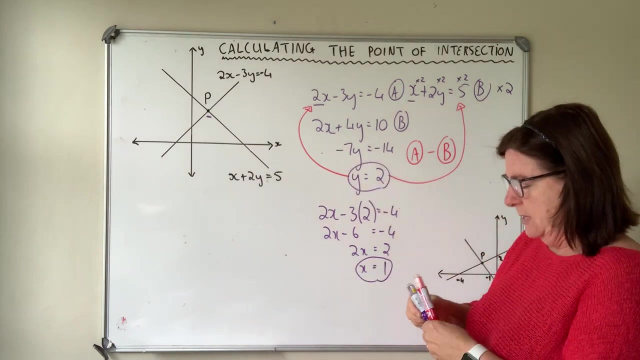 So 2x minus 6.. So 2x is 2.. So x is 1.. I'm moving quickly because I think this is easy for now. So therefore I have my answer: x, 1,, y, 2.. So if we put it as a point, 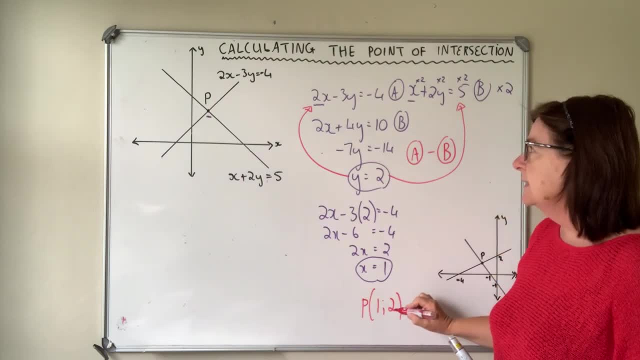 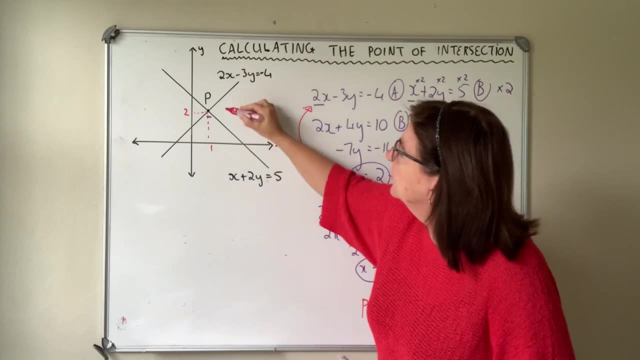 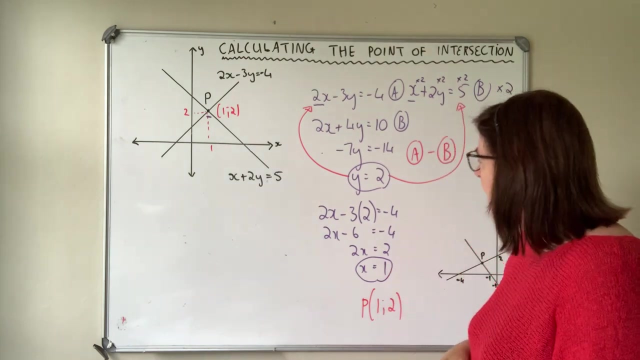 point P is going to have 1, 2.. Let's see if it ties up with our sketch. It looks more or less like it should be the point 1, 2.. Remember, it's never drawn to scale. Now, in this particular example, they gave us the equations of the straight lines. 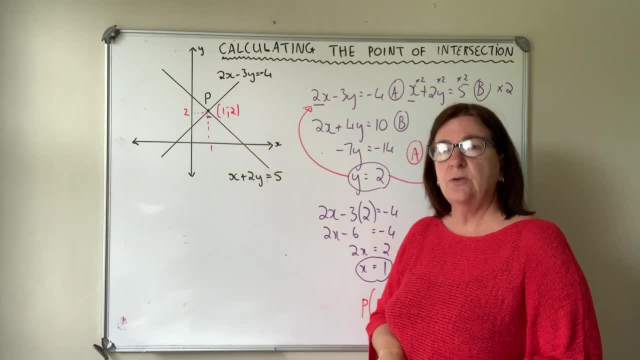 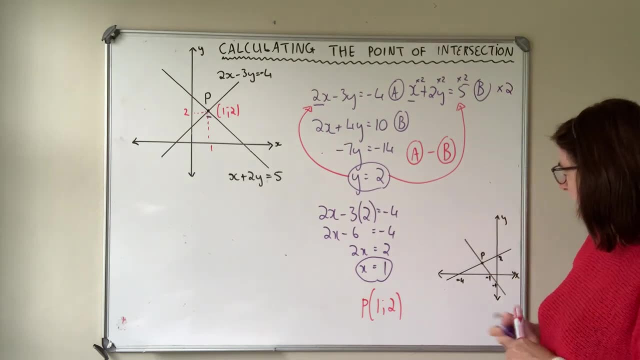 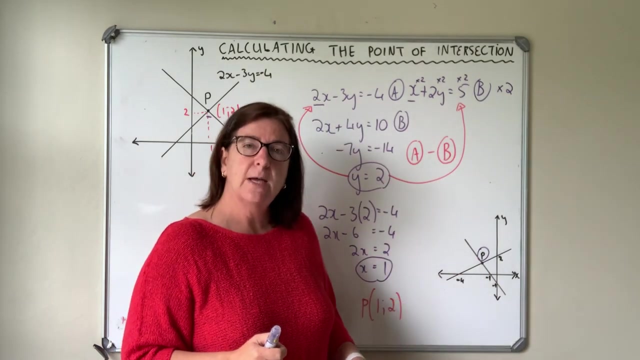 there and there, But in some examples that you're going to be doing now on your own- for example, this example over here- you need to find point P, But there are no equations given, But there are facts given. So what we need to do first is to 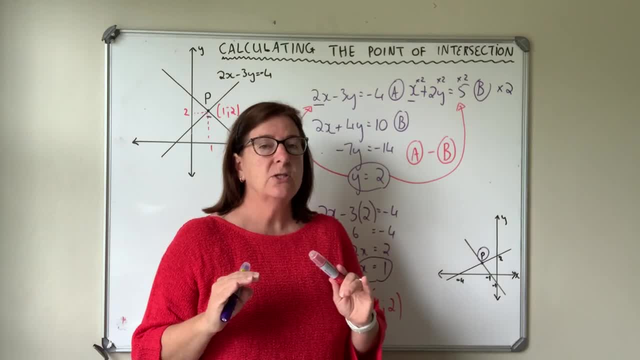 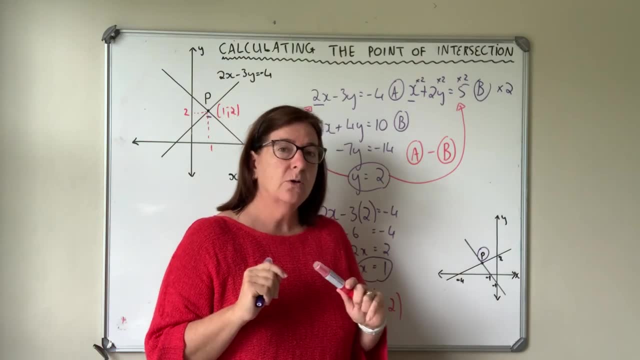 find the equations of the straight lines. Once we've got the equations of the straight lines, we can then solve for x and y using simultaneous equations. So remember, using yesterday's work, you're now going to find the equation of that line. You've got two points And to find the 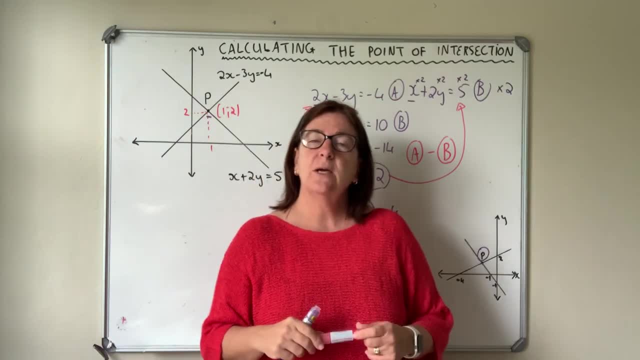 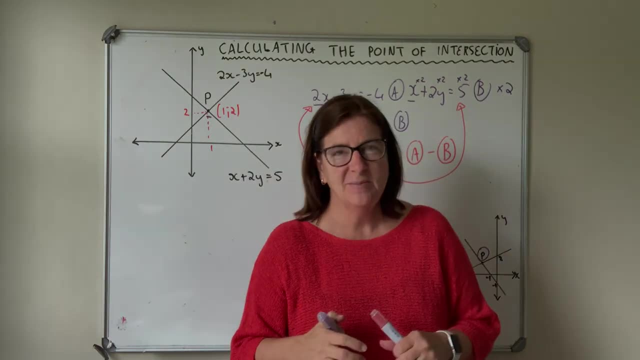 equation of that line. you've got two points, So we can find the equation of the lines, and then point P, which is the point of intersection. Good luck, grade 11s. See you soon. 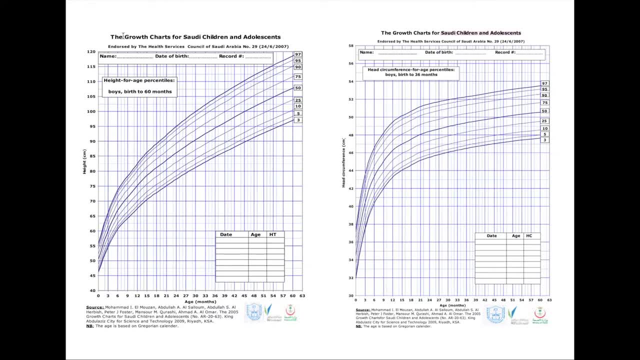 hello everyone. so today I'm gonna explain to you growth chart. it's super simple and easy. I'm gonna show you a different type and I'm gonna give you some example. so first thing you could check, and growth chart. you will check the nationality. as you see here, it's for Saudi. the region I have this chart is 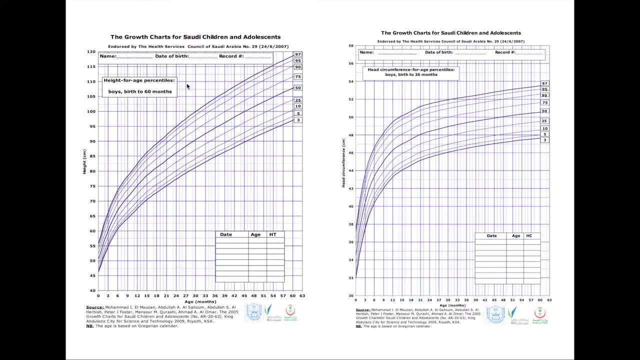 for Saudi children and adolescents. this is the first thing you can. you can check. where is it from? number two, you will check. what is it like? is it measuring the height, the head circumference? also, it's always like this: a play and white boxes, like here. like here, you can see it. so here I had first had circle.